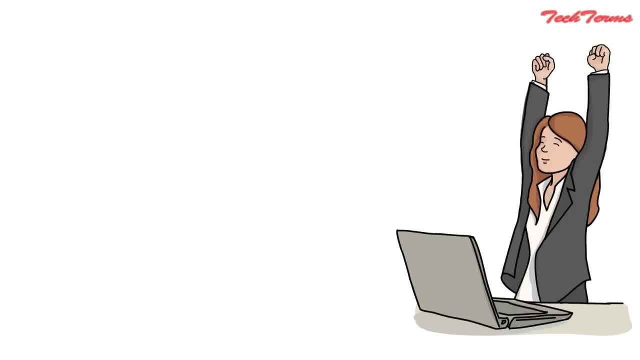 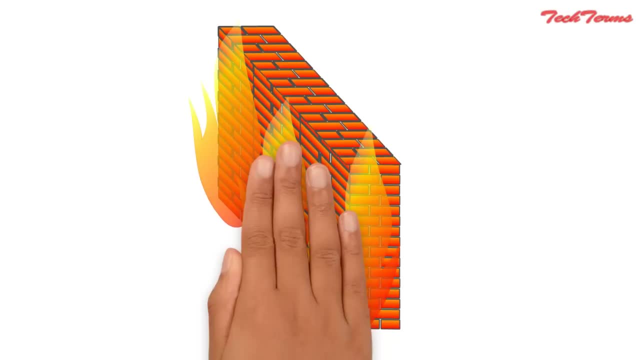 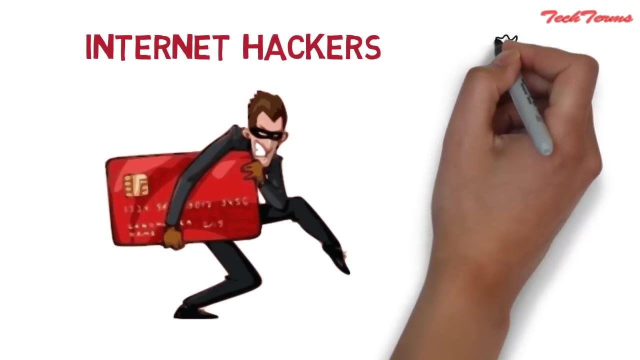 Hey guys, this is DG. Today, we are going to understand different types of firewalls and decide which firewall will best suit you as per your implementation environment. So let's start. Firewalls protect our computers from internet hackers. Internet hackers can steal our bank details from our computers and can reduce our bank balance from thousands of dollars to zero within seconds. 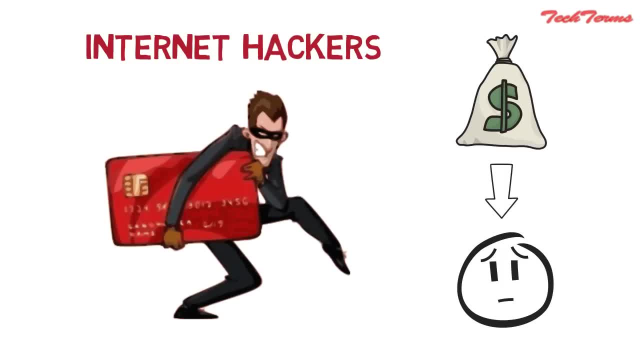 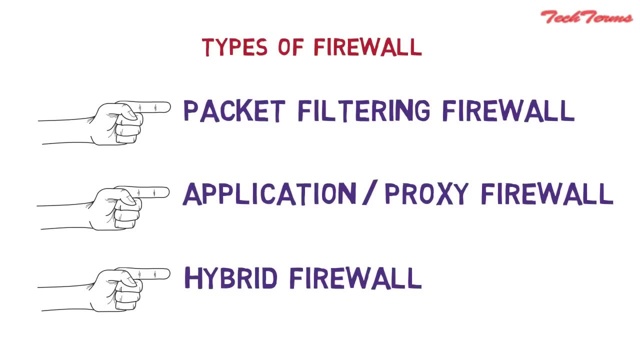 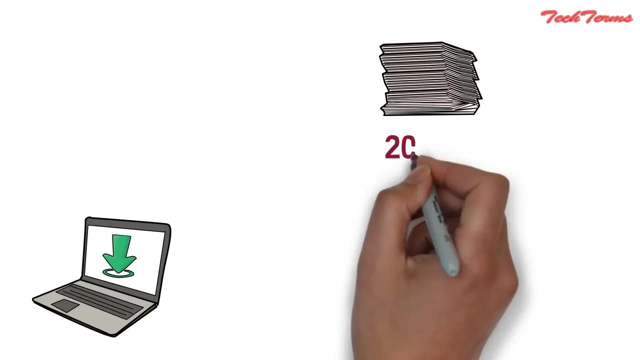 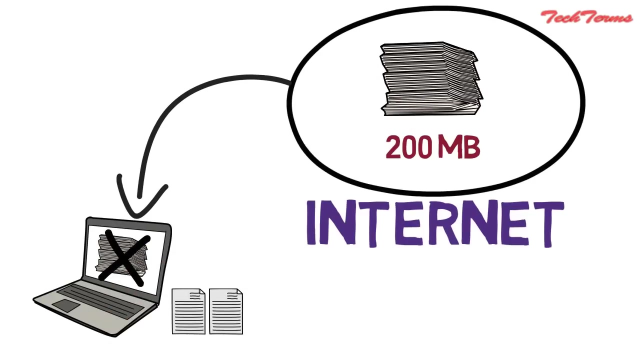 So firewall is a must in a computer or in a computer network. There are three types of firewalls: Packet Filtering, Firewall Application or Proxy Firewall, and Hybrid Firewall. Before starting with firewall types, you should know what are data packets. When we want to download a file of size, say 200 MB, from internet, then we will not receive the entire 200 MB data at once, but we will receive small packets, say 5 MB every second. 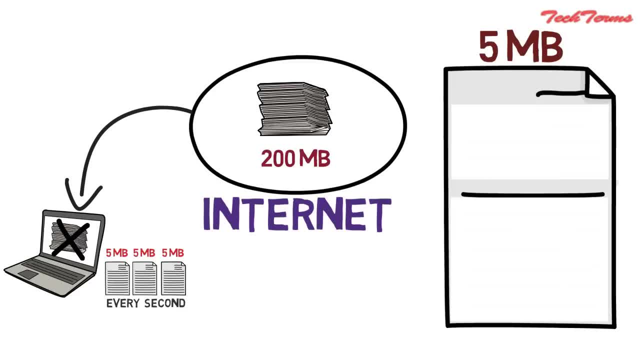 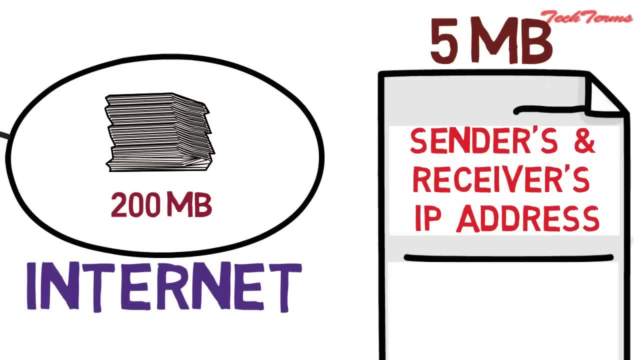 Some of the part of this 5 MB packet is occupied with information like which computer is sending the data, which computer is sending the data, which computer is receiving the data, etc. The remaining portion of this 5 MB packet contains the part of the actual data that we want to download. 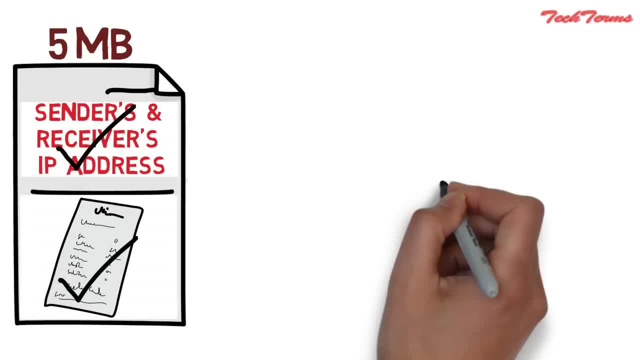 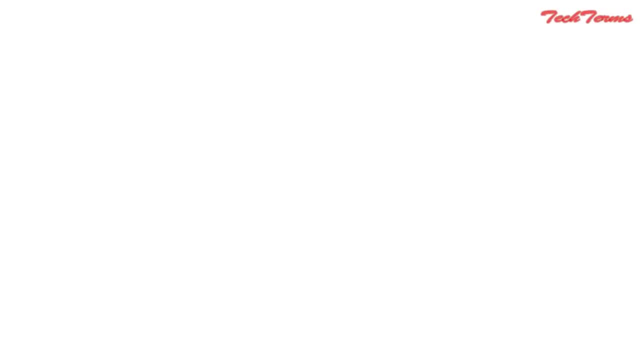 So part of the actual data plus some information together forms a data packet or IP packet, And this part of actual data is called payload. Now we can start with firewall types, Starting with Packet Filtering Firewall. Suppose I am downloading a file from internet. 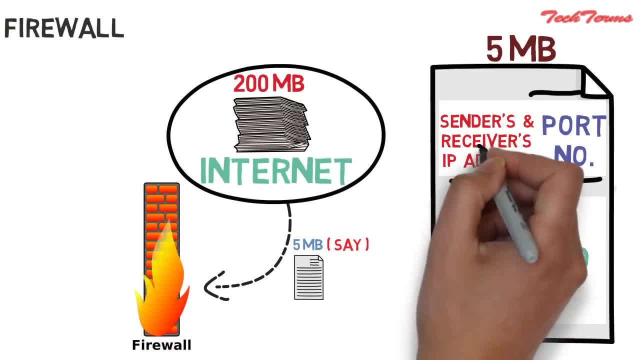 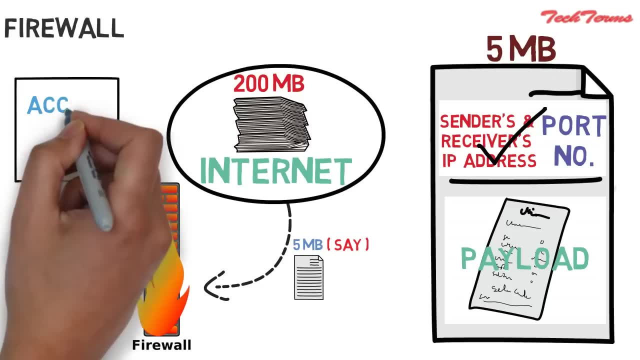 When the data packet arrives, a Packet Filtering Firewall. it only checks the senders and the receivers. It also checks the receivers IP address and the port number present in the data packet. The rules written in a list called Access Control List are used for data packet verification. 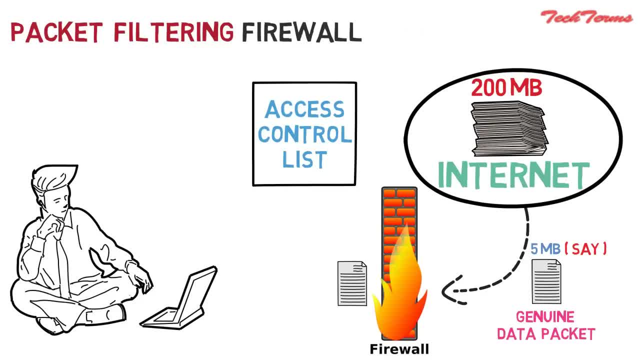 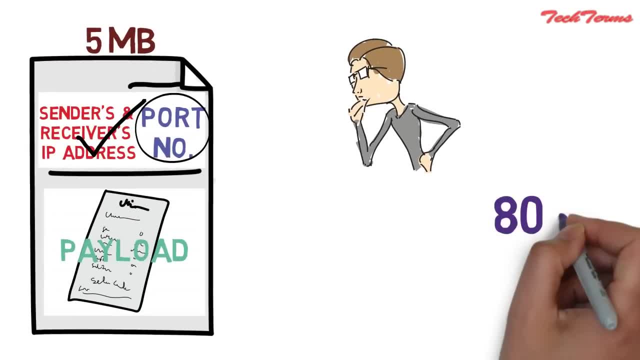 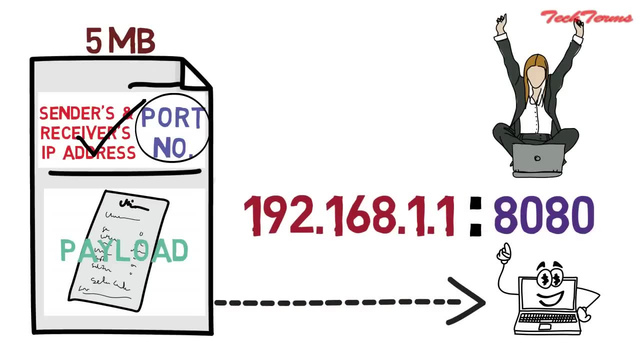 If everything is OK, then the data packet is allowed to pass through Packet Filtering Firewall and then to my computer. But what is port number? Actually, these are some digits written after IP address, separated with a colon, and are used for the successful data packet transfer. 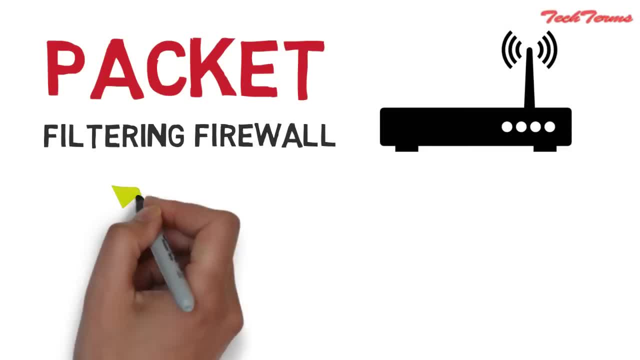 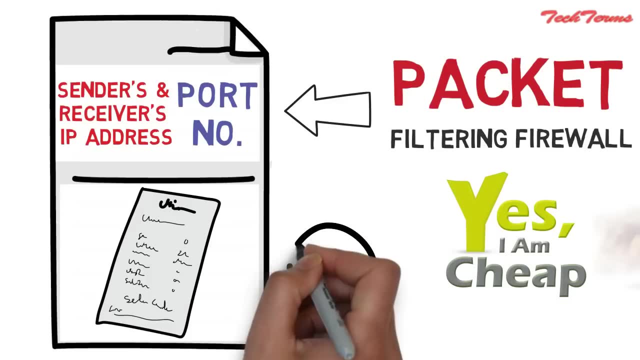 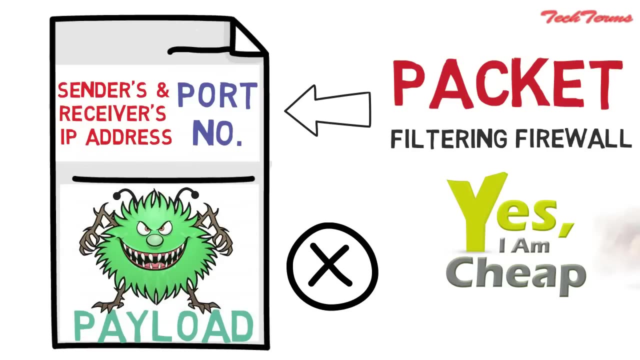 The Packet Filtering Firewall is already present in internet routers, So they are the cheapest and the quickest way to implement. The only limitation of Packet Filtering Firewall is that it do not checks the data portion that is payload of the data packet, So a hacker could send some malicious data packed in this payload section. 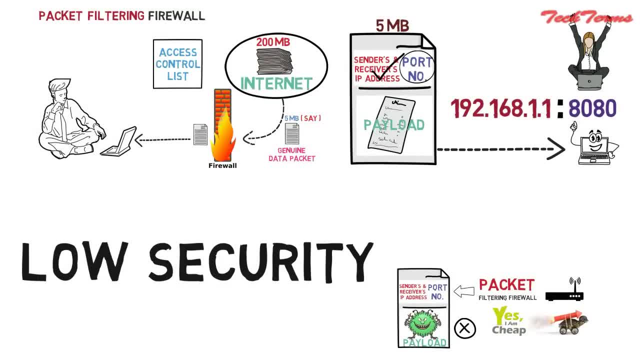 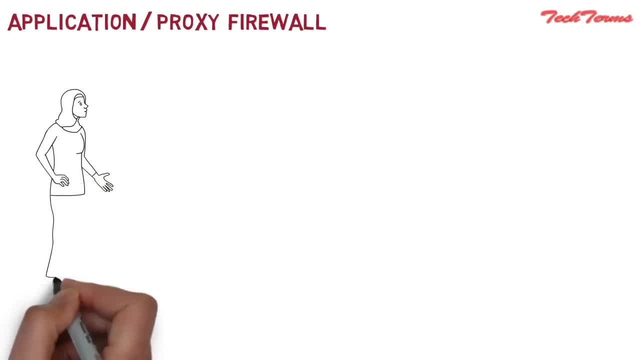 Hence Packet Filtering Firewall provides low security. The second one is Application or Proxy Firewall. Let us understand it with an example. Suppose your mom asks you to buy a pen from the market. You go to the shop, buy the pen. 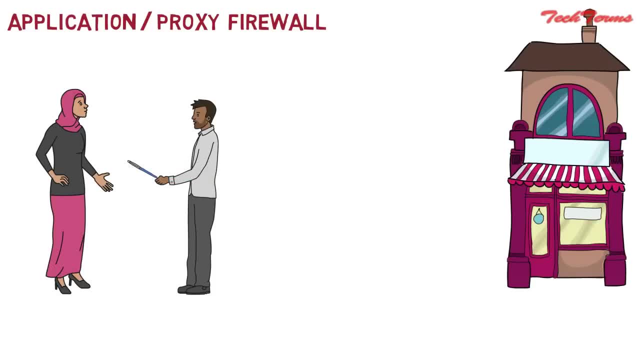 come home back and give the pen to your mom. Here you had done the work that your mom wanted you to do, without letting the shopkeeper knew who actually wanted that pen. Same is the case with Application or Proxy Firewalls. Replace the shopkeeper with internet. 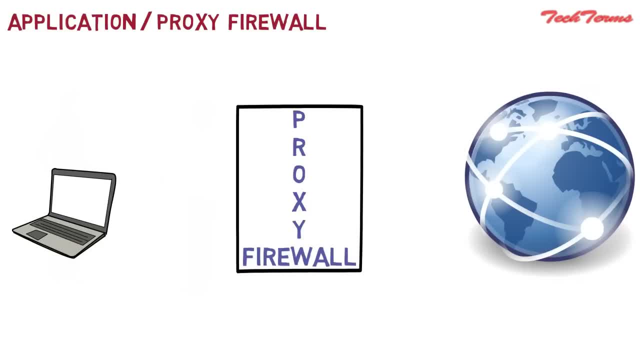 your mom with personal computer and yourself with Proxy Firewall, Like you did not let the shopkeeper knew that your mom was the one who actually wanted that pen. Similarly, Proxy Firewalls do not let the internet know which computer actually wants to visit the requested website. 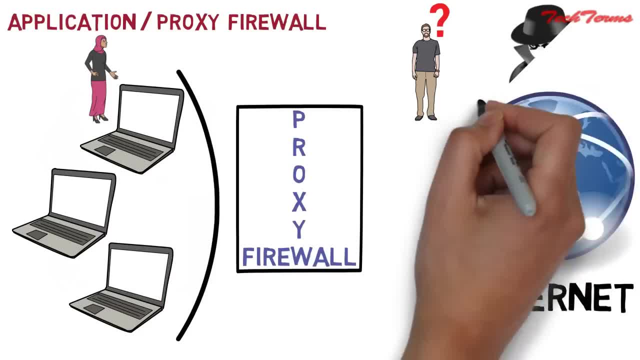 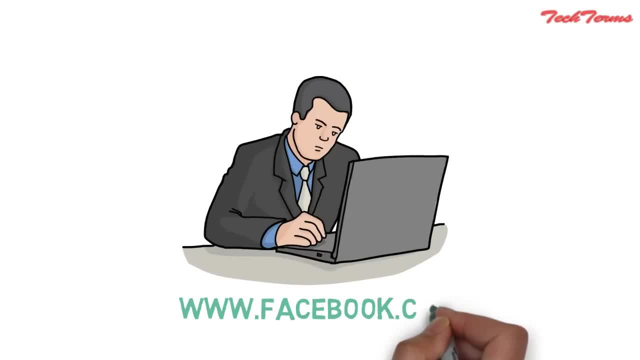 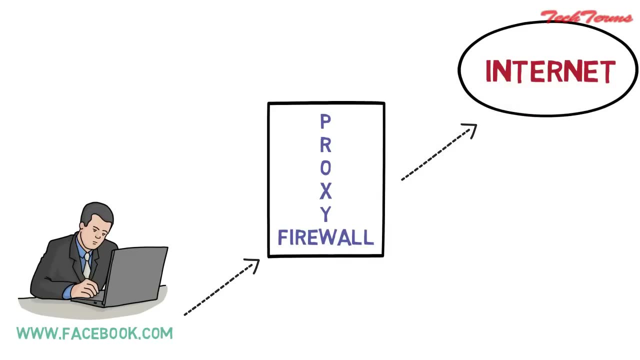 That is, Proxy Firewalls- hides us from attackers in internet. Let us understand this whole process. User enters the website wwwfacebookcom in the web browser. Proxy Firewall receives the request and forwards that request to internet. The web server in internet receives the request. 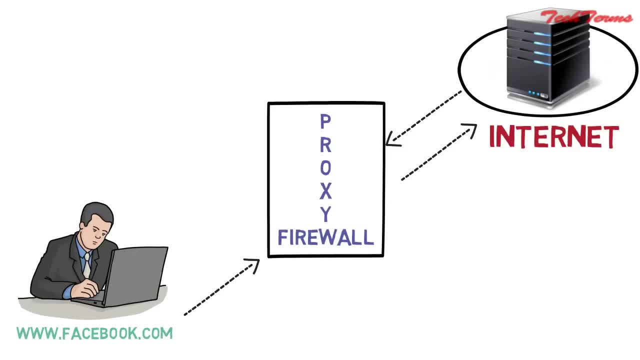 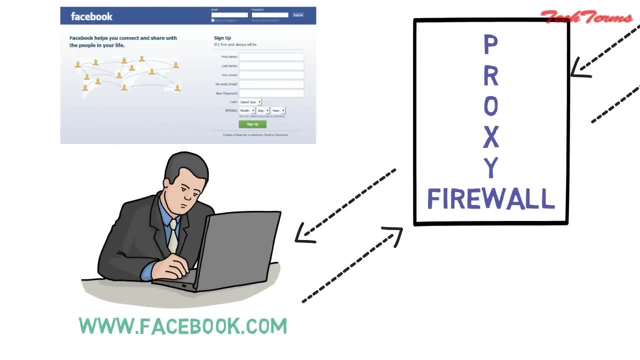 and responds back to the Proxy Firewall with the requested information. The Proxy Firewall receives the information and forwards it to the original client for his viewing pleasure. In this whole process, web server thinks that Proxy Firewall is the one who wants to visit wwwfacebookcom. 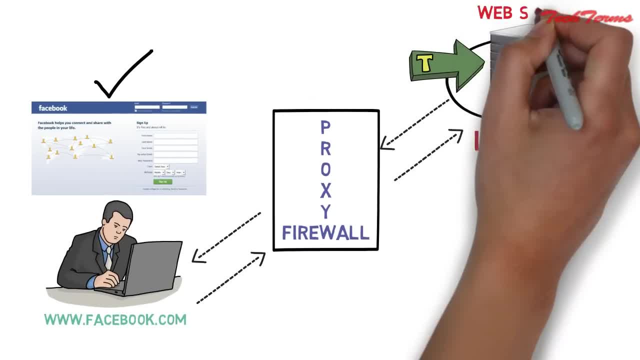 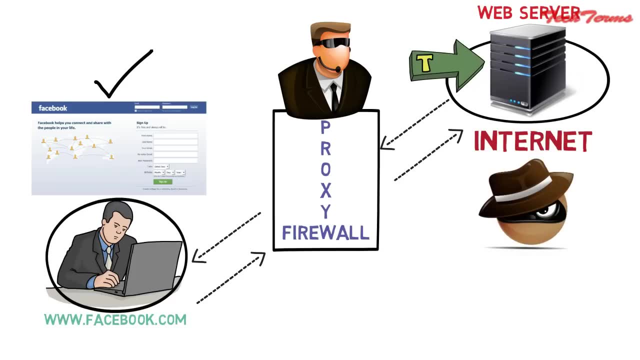 That is, Proxy Firewalls do not let the web server know the origin of the request. So Proxy Firewalls protect us from the potential attackers in internet by not disclosing our computer's identity, or I should say by not disclosing our computer's IP address. 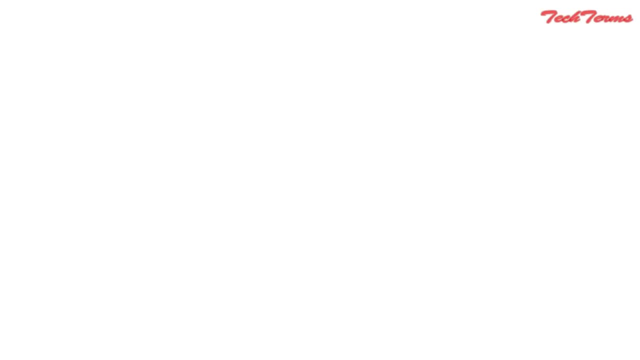 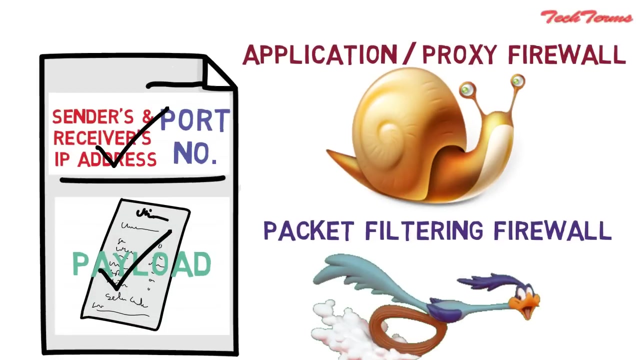 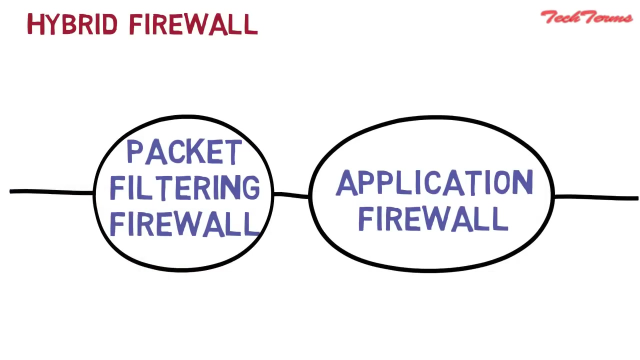 Since Application Firewalls also check the payload of the received data packet, so they are generally much slower than the Packet Filtering Firewalls. Third is Hybrid Firewall. Hybrid Firewalls combine Packet Filtering Firewall and Application Firewall in series to enhance the security. 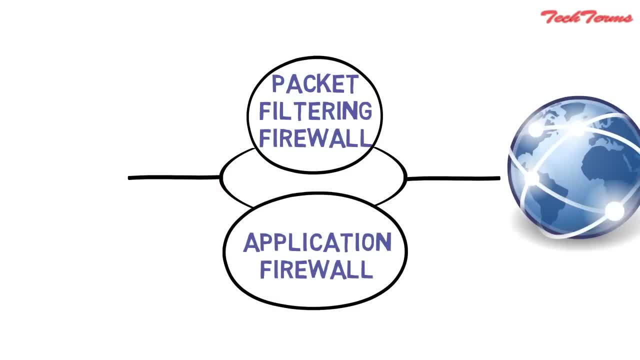 If they are connected in parallel, then the security of the connection will be reduced to the parameters defined by Packet Filtering. Firewall, That is, Application Firewall, will be of no use if the two Firewalls are connected in parallel. For this reason, Hybrid Firewalls use Packet Filtering.